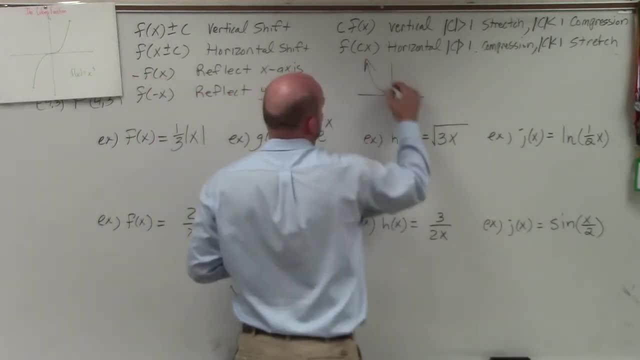 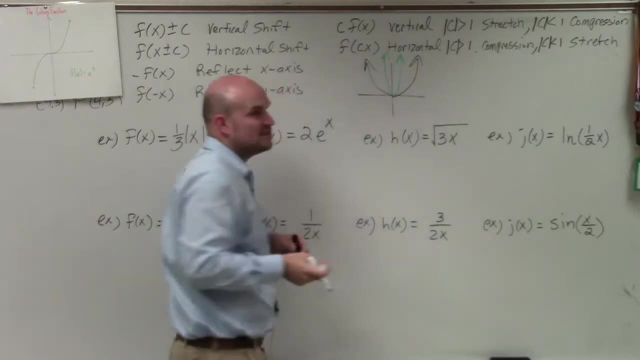 But if you guys remember when we were doing quadratics, remember when we did a stretching and compressing, It looks something like this, right, So think about it. I mean, a vertical stretch is the same thing as a horizontal compression. 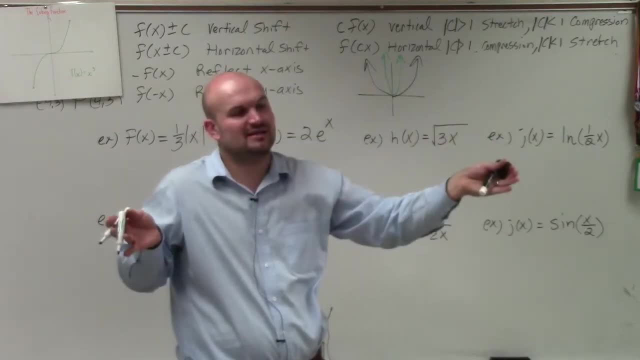 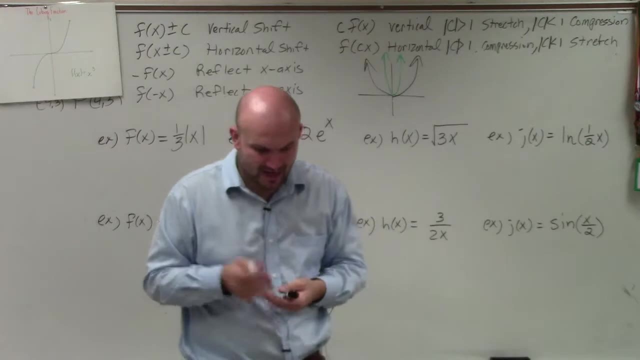 That's why these are kind of opposite. Whatever you vertically stretch is like the horizontal compression, So those kind of get swapped around. Anyways, what I'm going to do Is let's first identify: am I multiplying a value inside or outside? 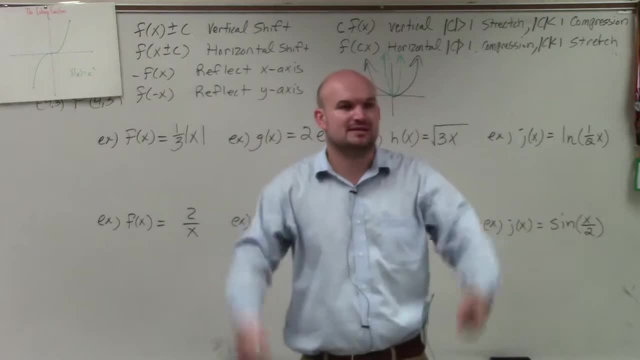 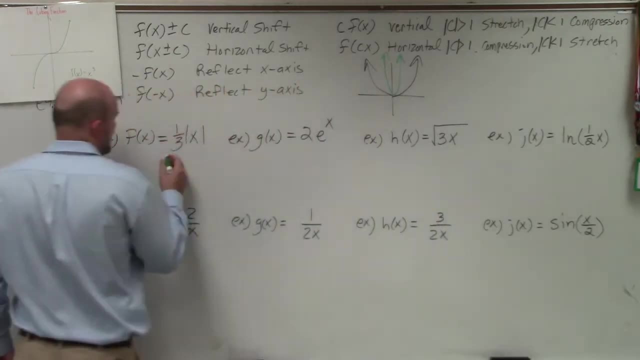 I think if you guys can get that, then you can just follow these rules And we'll just practice these over and over. Yes, So can we do the parent function first? if we don't understand, Sure, we can do the parent function. 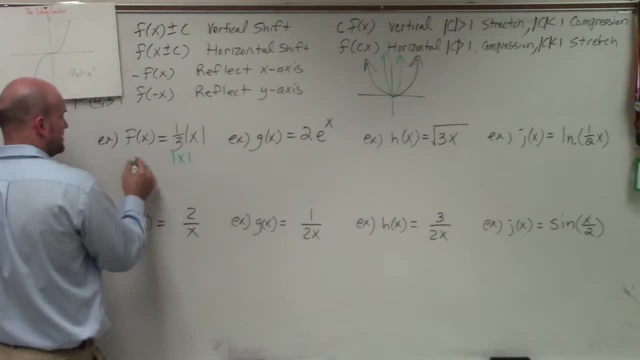 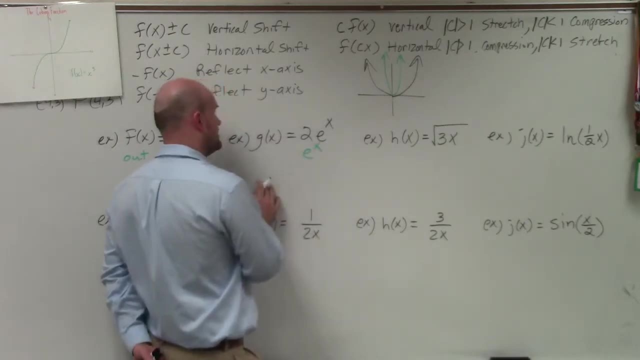 Parent function over here is absolute value of x. Am I multiplying it on the outside or the inside? I'm just going to write out, or in The parent function. here is e to the x. Am I multiplying inside or outside? Outside? Here parent function is square root of x. 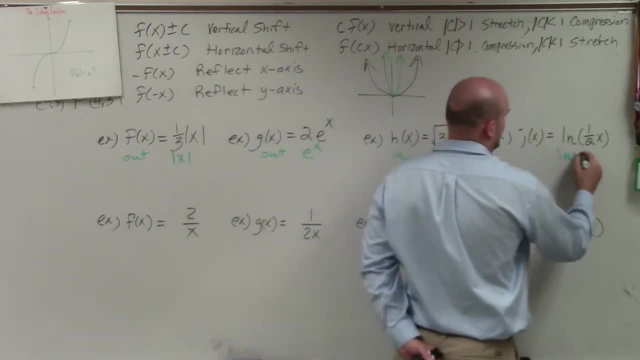 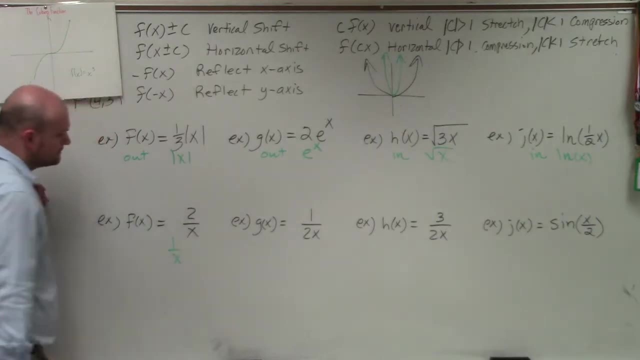 I'm multiplying by the inside. Here my parent function is ln of x And I'm multiplying by the inside. Here I have 1 over x Outside- Outside. You could say: yeah, it's technically. I'll show you. 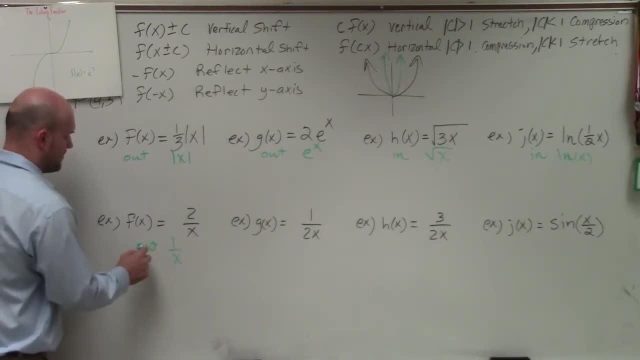 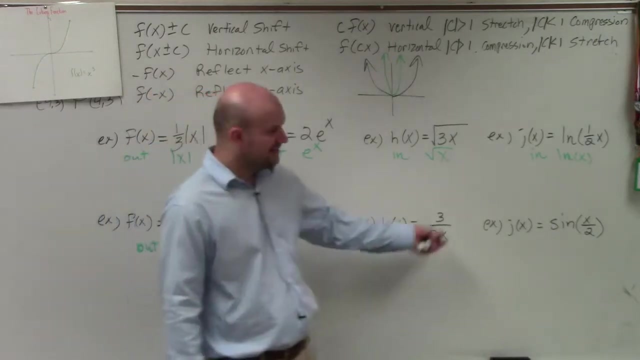 but it is going to be outside Technically, but I'll show you. It kind of could get out of the way, But you could say that this would be in and 1 over x And this one is. you could say it's kind of like both. 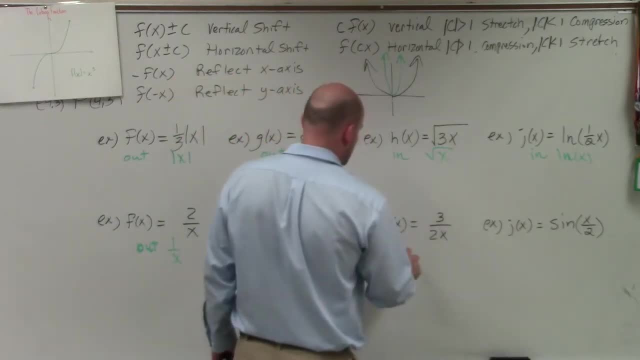 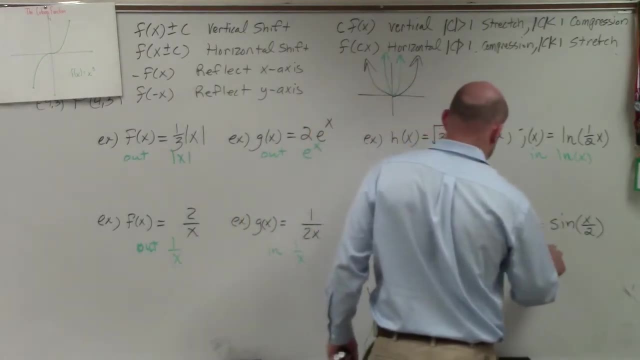 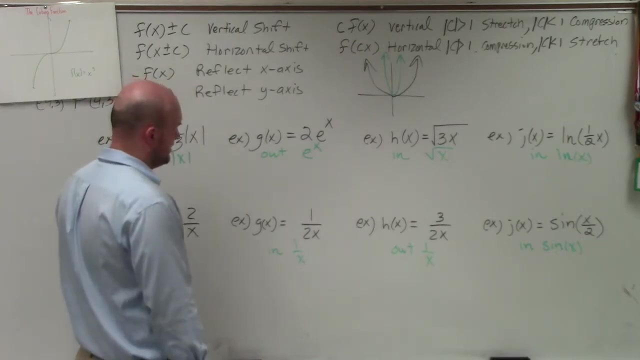 You're multiplying by both of them, right, But I'm just going to say this as an outside and I'll show you why. And then over here in, And it's really technically doing the exact same thing. Well, here. 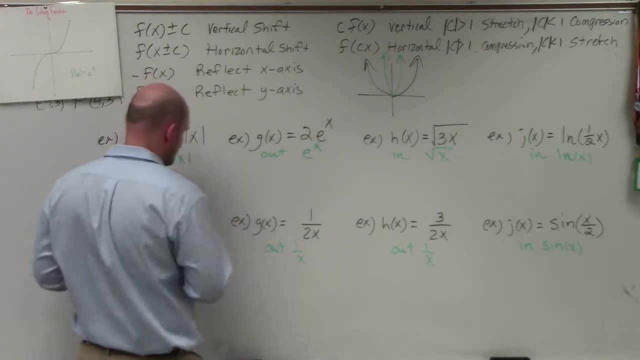 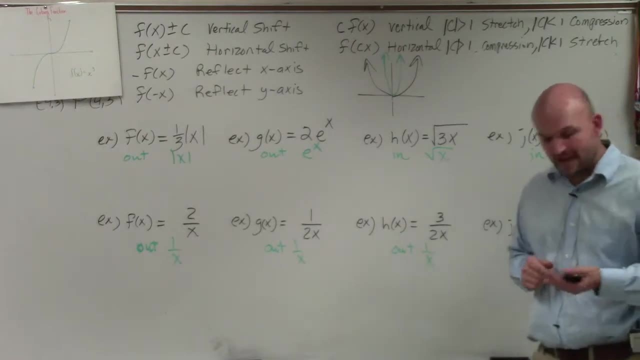 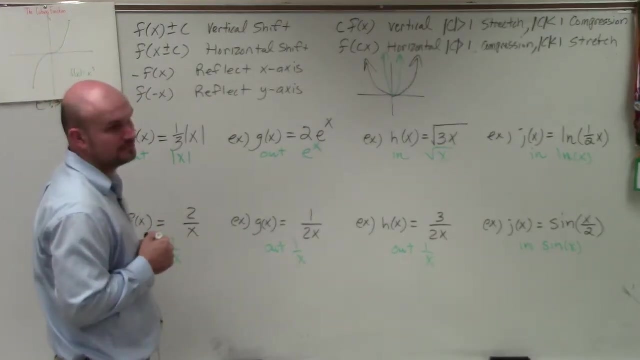 Let's just make this All the same. Let's just make this all out And I'll just explain why. OK, So now let's go through it. So I'm multiplying out. So therefore it's: the vertical Is 1 third greater than 1 or less than 1?? 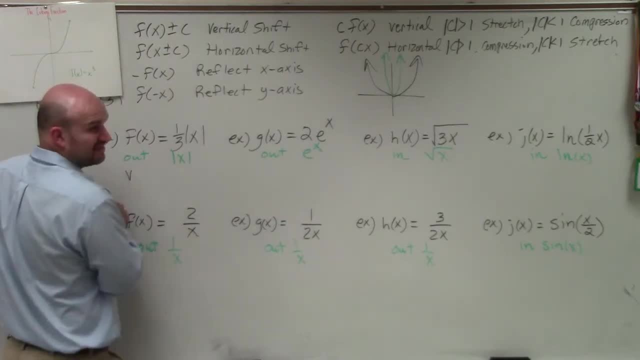 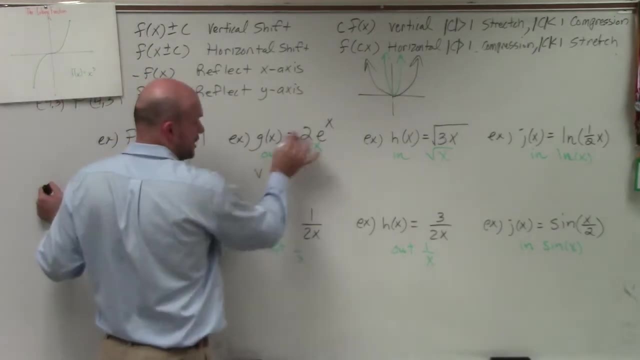 Less than 1.. So therefore it's a. I'm just going to write v because I'm trying to move along compression. This is outside, but it's larger than 1. So it's a vertical stretch, OK. 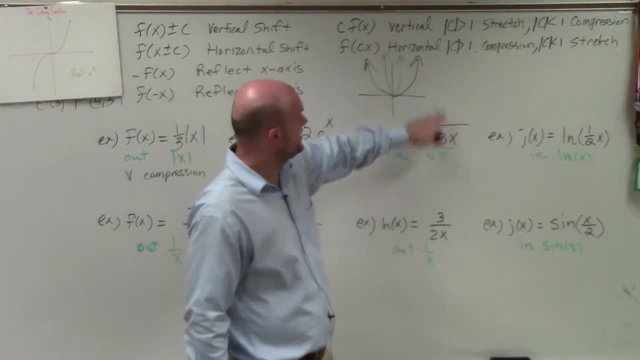 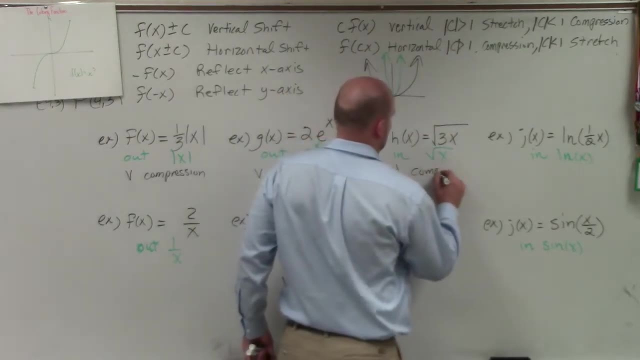 Over. here I'm multiplying by the inside, So it's horizontal. 3, absolute value of 3 is greater than 1.. So it's a horizontal compression Here I'm multiplying by the inside, But it's less than 1.. 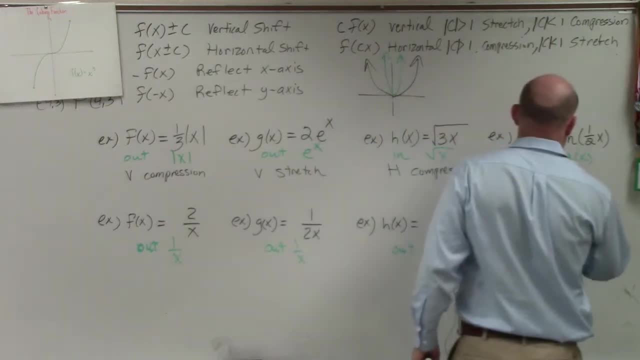 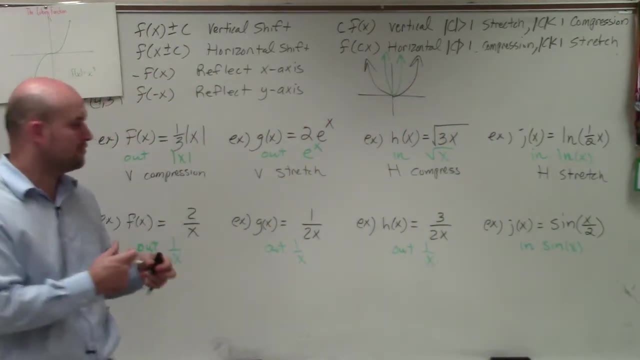 So it's a horizontal stretch, And having your notes available when you guys are doing your homework will be helpful Because, again, you were just going to practice. We're going to practice over and over in these, So therefore we can eventually kind of get used to them. 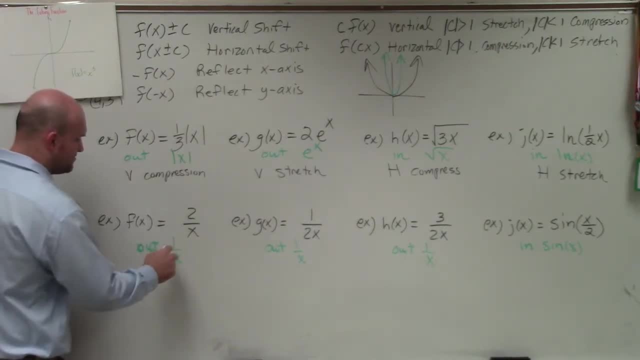 Now the reason why I wrote this as outside: because, ladies and gentlemen, I could just multiply the parent function by 2.. Would you guys agree? So, technically, you're just taking this function and multiplying it by 2. So therefore, we can call it outside. 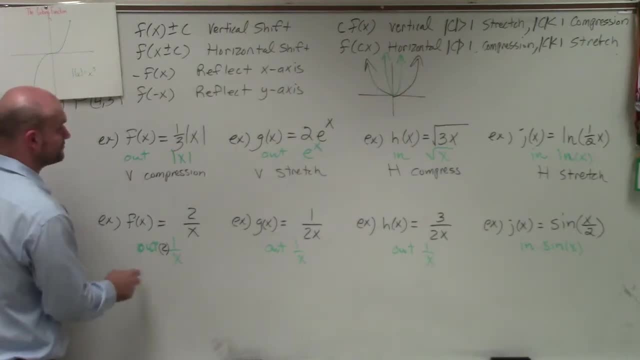 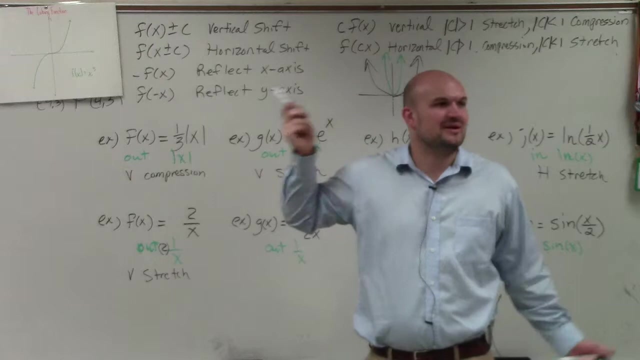 So therefore we could say it's a vertical stretch because 2 is greater than 1.. Now the reason why you could have done in or out outside of these, because 1 over x is an odd function, So it actually it can go either. 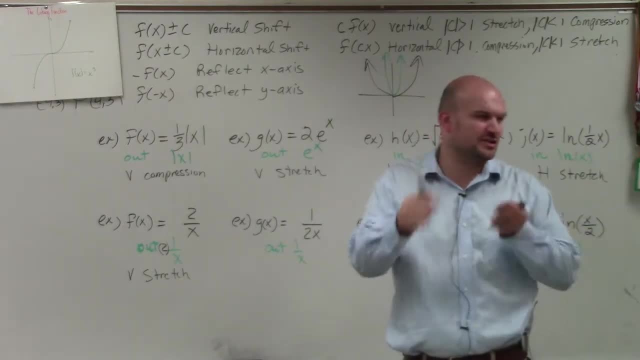 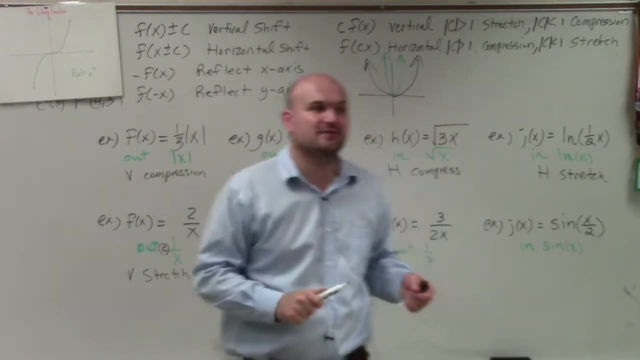 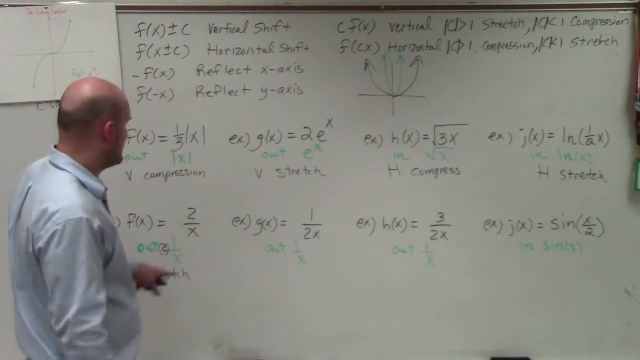 It doesn't actually matter if it's vertical or horizontal, It's actually either, or because it's an odd function. The same thing works for the identity function. By shifting it to the right, it's the same thing as going up Or as going down. sorry, 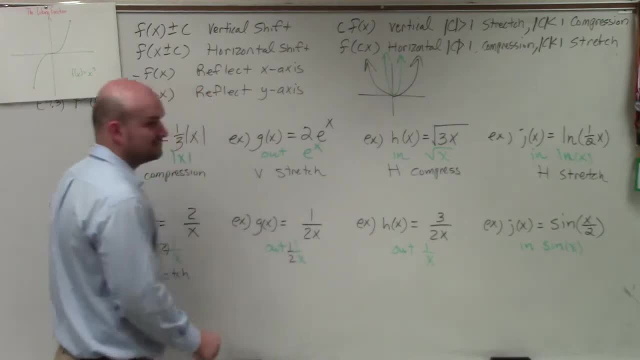 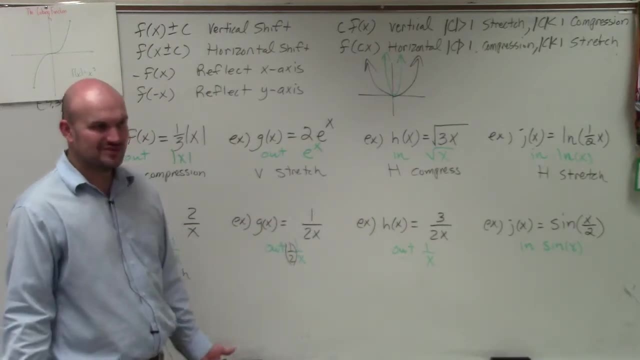 So this one. I could rewrite this as multiplying it by 1 half. right, I could factor out the 1 half Because what's 1 half times 1 over x, 1 over 2x, So therefore the outside, that's fraction. 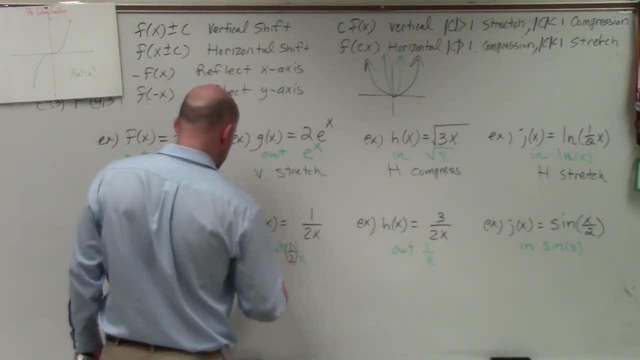 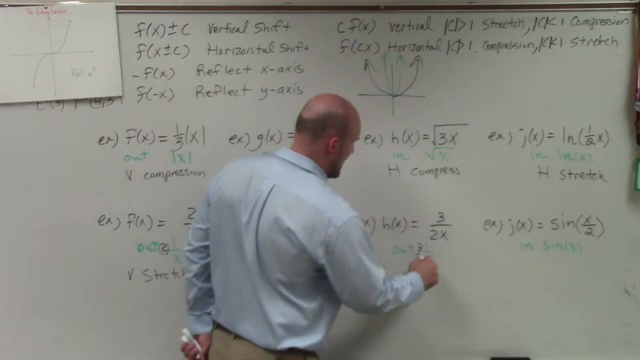 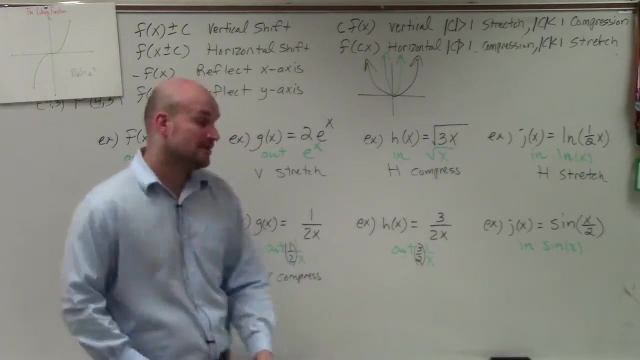 So therefore you could say that it is a vertical compression. Over here I could factor out a 3 halves. So now, 3 halves is a fraction, But is 3 halves less than 1 or greater than 1? Greater than 1.. 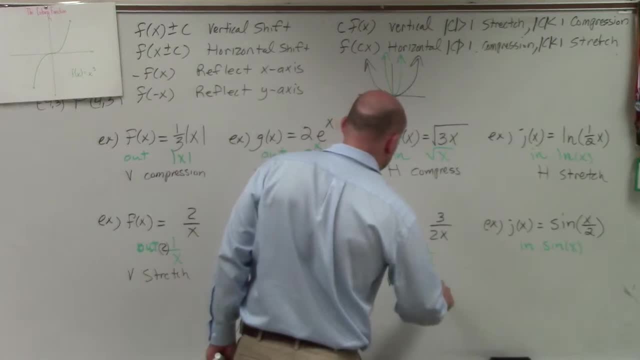 So, therefore, this is a vertical stretch, And then this last one. this one confuses a lot of students And we're going to get into this much more later in the year, But you can rewrite this as sine of 1 half times x. 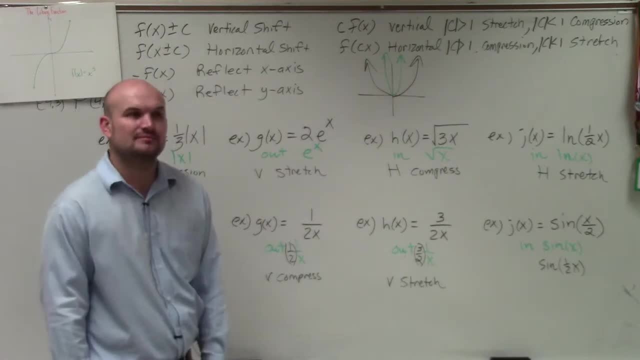 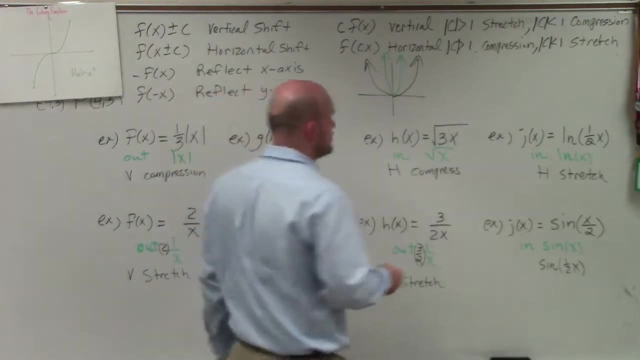 Because what's 1 half times x? x over 2. It's the same thing, right? So therefore I'm multiplying by 1 half. inside the function, 1 half is less than 1. So it's a horizontal stretch. All right. 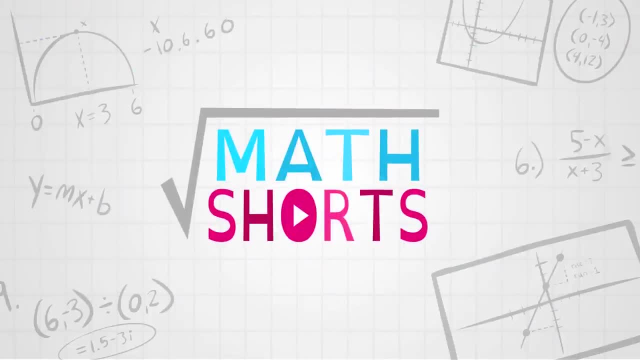 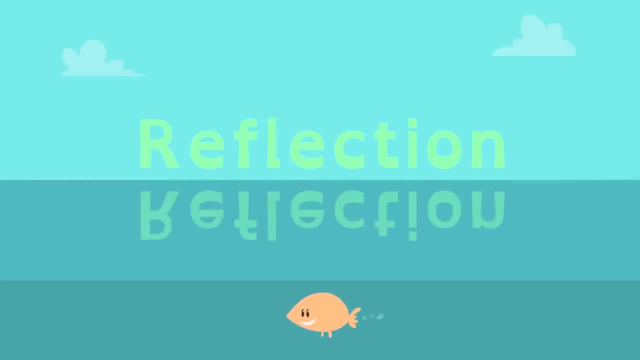 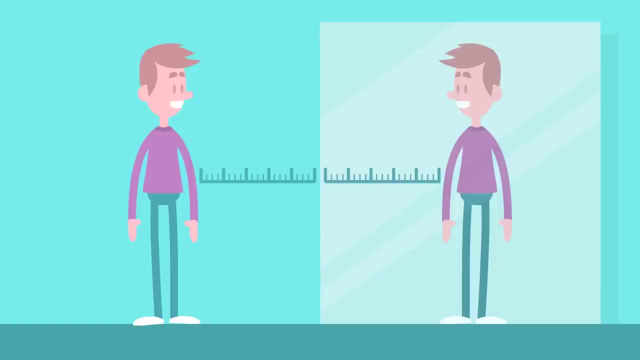 Reflection is a type of movement or change in a geometric shape. Think about when you look in a mirror. You see a reflection of yourself. See how your reflection appears to be the same distance from the surface of the mirror as you are. Also note how the left and right sides are reversed. The same is true with geometric shapes. 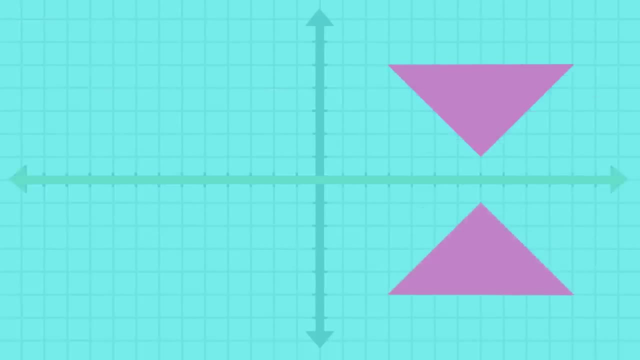 When we reflect this triangle like this, the x-axis acts like a mirror. You can reflect all kinds of shapes as long as you determine the line that you want to reflect on, just like a mirror. For example, you can use any line along the x-axis or the y-axis. 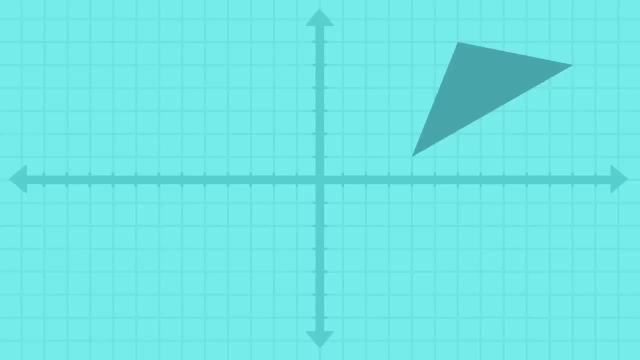 You can even reflect a shape through a line using an expression such as x equals 1.. In this example, the line x equals 1 is the line of reflection for the two triangles. You can use any expression to create a line of reflection anywhere. 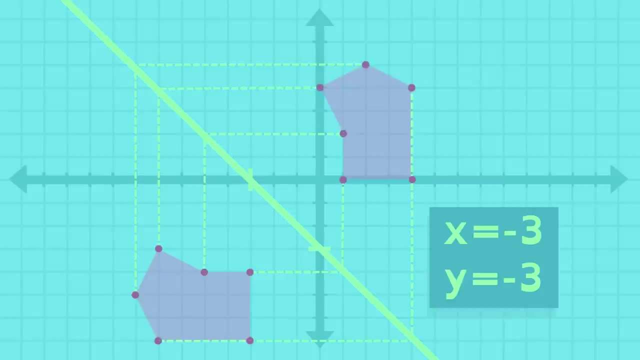 The way to make sure a shape is correctly reflected is to check that each point of one shape is the same distance from the line of reflection as the corresponding point in the other shape, and that it has corresponding sides and corresponding angles, Just like other transformations. you can record the coordinates of the shape and its image to demonstrate the reflection too. 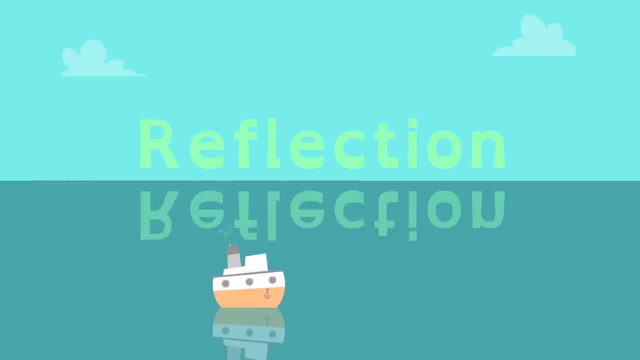 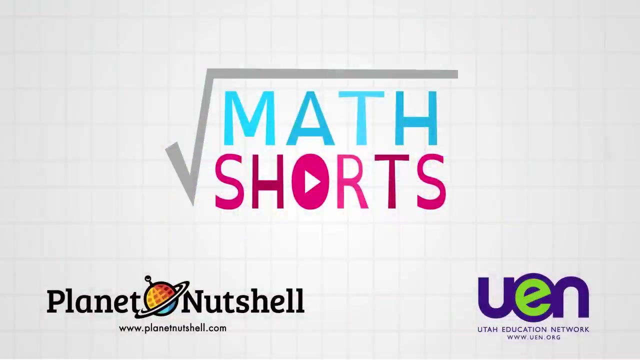 Reflection makes a mirror image. It's one type of movement for geometric shapes, So we can use a mirror image of these three same shapes and try to suggest the form of a mirror. Let's go back to the paper plate. We'll look at the two shapes we just created.